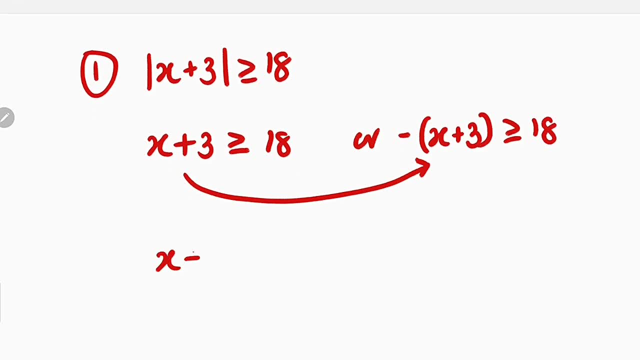 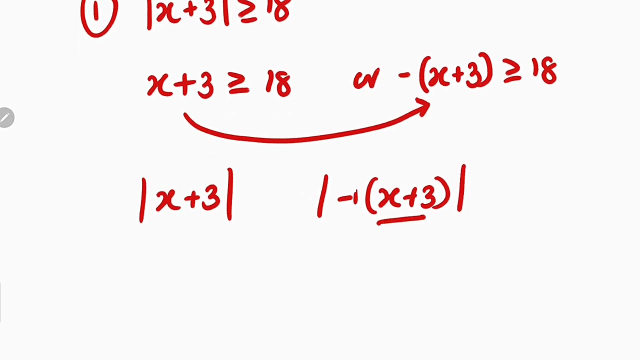 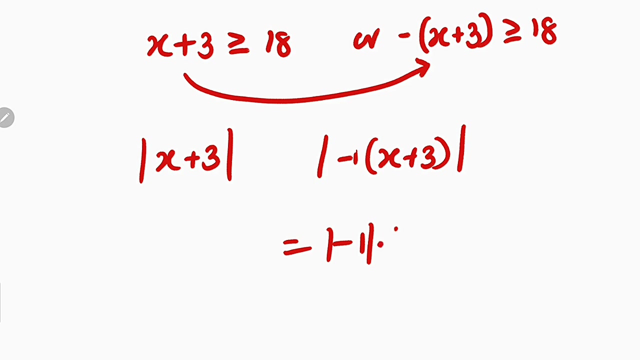 Let me give you an instance. If you have absolute value of 3x plus 3 and you also have absolute value of negative, If you have absolute value of 3x plus 3 and you also have absolute value of negative, Did you know that since there is multiplication between this negative 1 and this, you can split the absolute value into the absolute value of negative, 1 times the absolute value of x plus 3.? 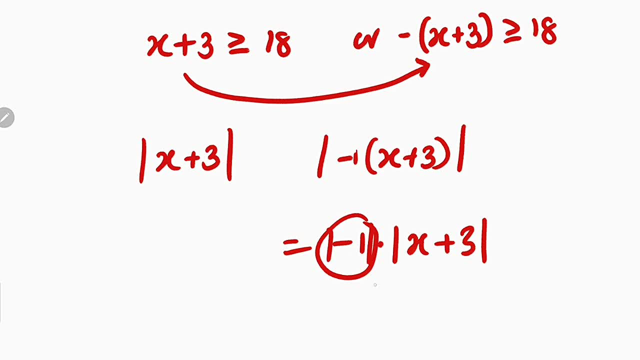 And the absolute value of negative 1 will be positive 1 times absolute value of x plus 3 will still be absolute value of x plus 3, which is the same thing with this one. So they are all the same. So from here you solve them separately. 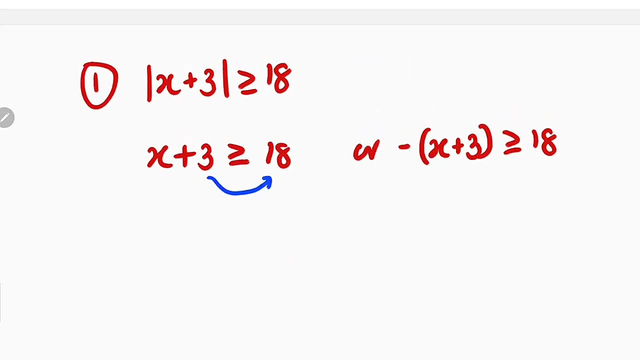 We have the first one. Taking this one to the other side, it becomes negative and 18 minus 3 will be 15.. So x greater or equal to 15.. Then you move to the other side. By multiplying both sides by negative 1, we have x plus 3 less than or equal to. 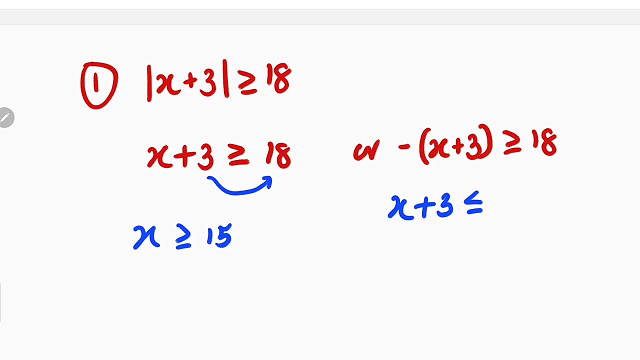 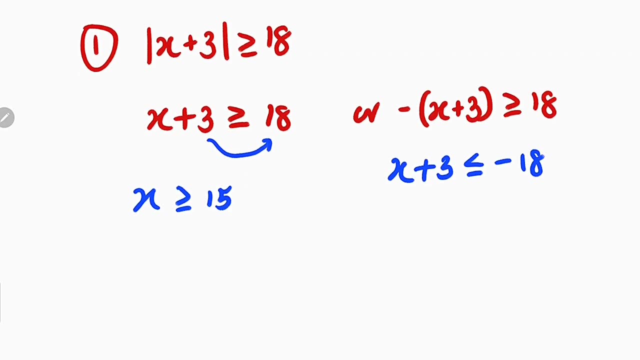 Remember, the direction of the inequality will surely change. if you multiply or divide both sides of an inequality by negative value, Then this becomes negative 18.. Take 3 to the other side, It becomes negative. So x will be less than or equal to what? 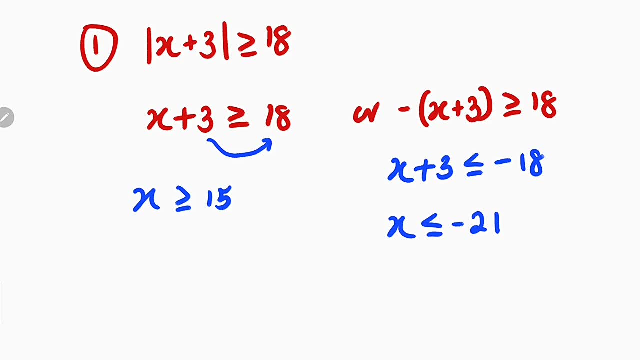 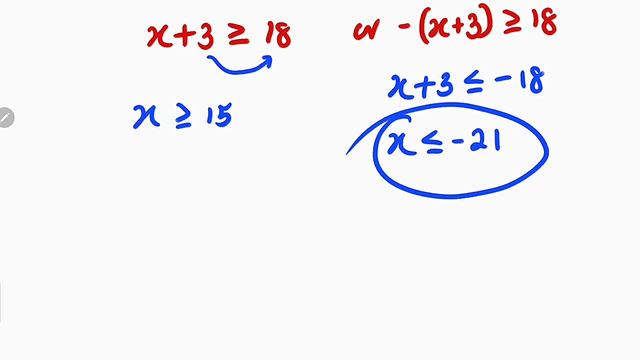 Negative 21.. So this is the solution to this problem, And you should know that values less than or equal to negative 21 is approaching negative infinity. You can also look at it on the number line: If you have 0 here, negative 21 will be here. 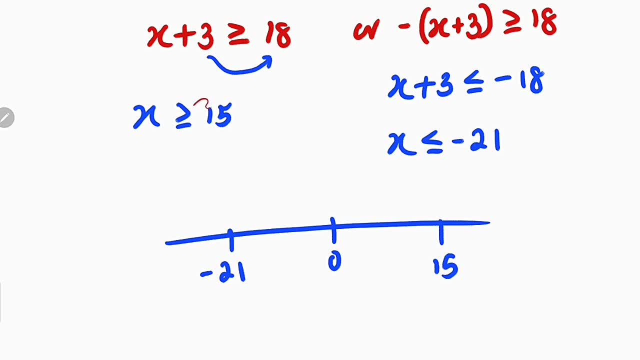 And we have 15 right here. So you can also look at it on the number line: If you have 0 here, negative 21 will be here, And we have 15 right here. So talking about values of x that are greater or equal to 15.. 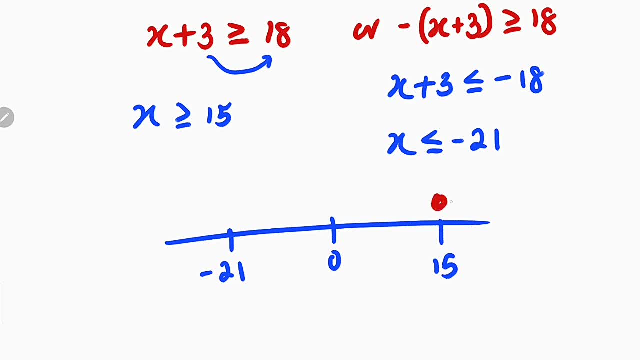 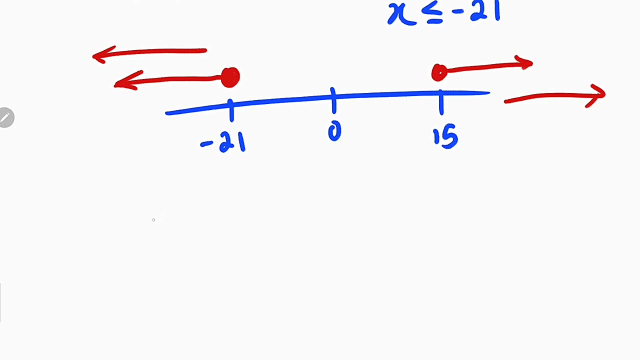 They are all values to the right hand side of what 15.. And values to the left-hand side of negative 21? So this is approaching negative infinity, while this is approaching positive infinity. So we can write it in an interval notation, as x belongs to the set of values from negative infinity down to negative 21.. 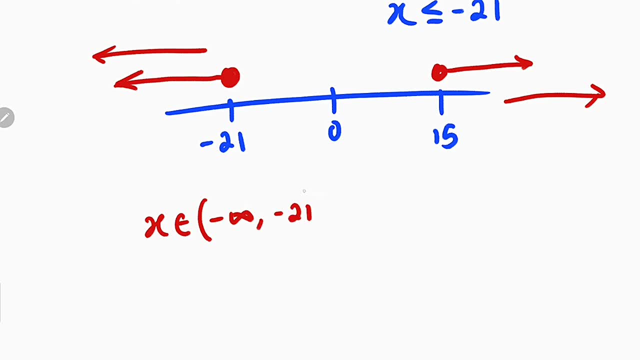 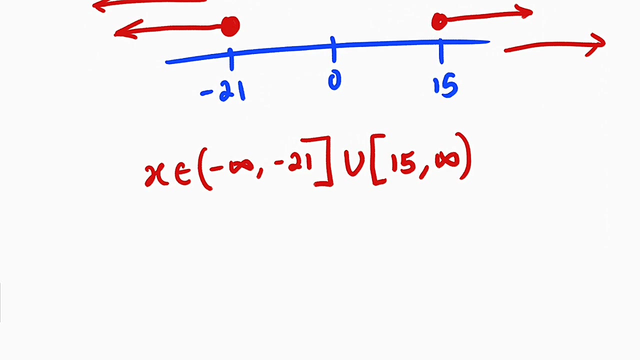 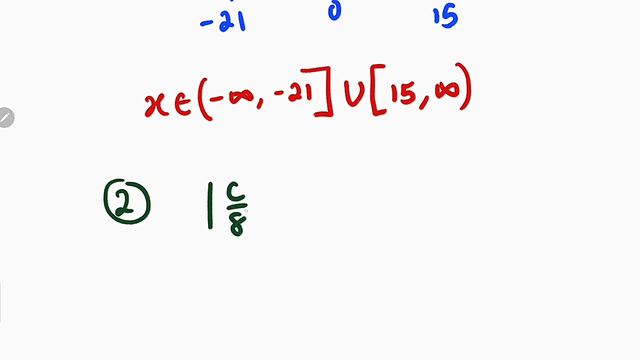 But negative 21 is still in many ones. Negative 21 is inclusive the union from 15 down to positive infinity. So this is just the solution in an interval notation. So let's take the second problem. Okay, problem number two: we are given that the absolute value of C divided by 8 is what? 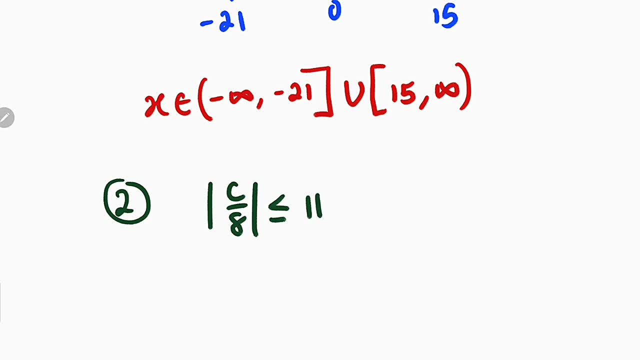 Less than or equal to 11.. So what you can do directly, you can say that this is the same thing as C divided by 8, less than or equal to 11. Then C divided by 8, you can mentally multiply both sides by that negative value directly. 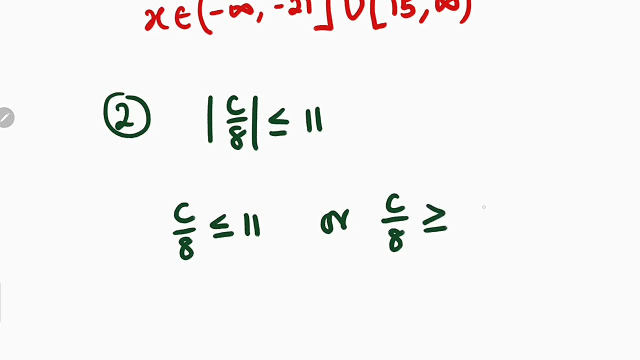 The direction of the inequality will change right. Then you negate this one, It becomes negative: 11. Then you solve: Multiplying both sides by 8, you have 7.. C less than or equal to 8,, 8.. 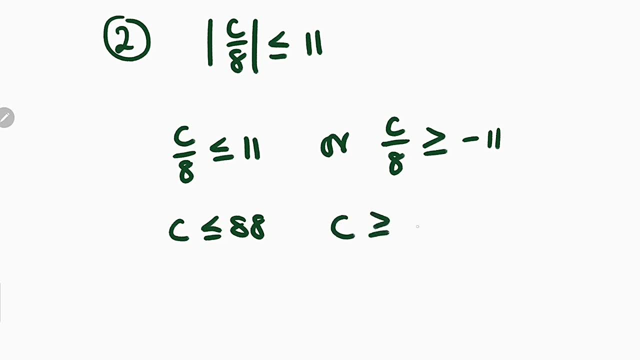 And we have C greater or equal to negative 8, 8.. So you can see that this solution is from negative 8, 8 down to 8, 8.. So this is what, In an inequality form, we have negative 8, 8 less than C less than okay, or equal to then 8, 8.. 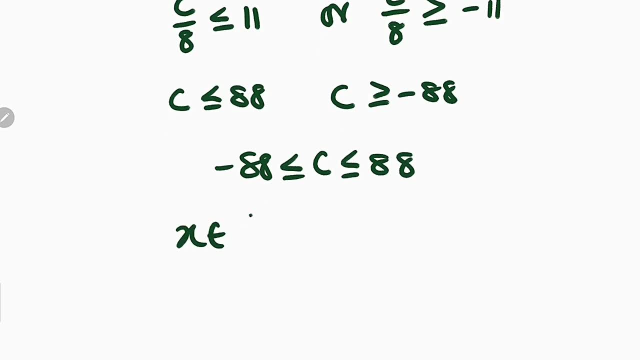 Or in an interval. notation X belongs to the set of values from negative 8, 8 down to positive 8, 8.. Let's take problem number three. Problem number three: we have the absolute value of 2M less than 16.. 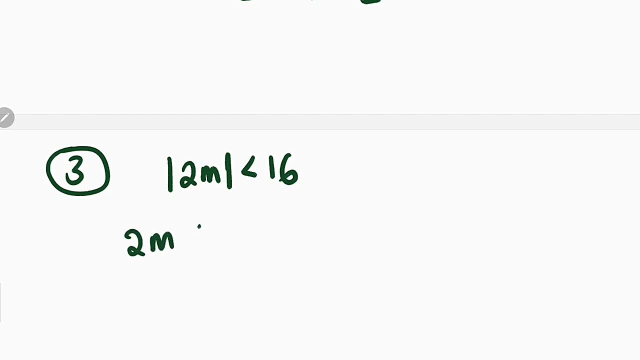 So we do the same thing: 2M is either less than 16 or 2M is greater than negative 16.. You divide both sides by: 2M is less than 8 or M is greater than negative 8.. So you see that the solution is what? 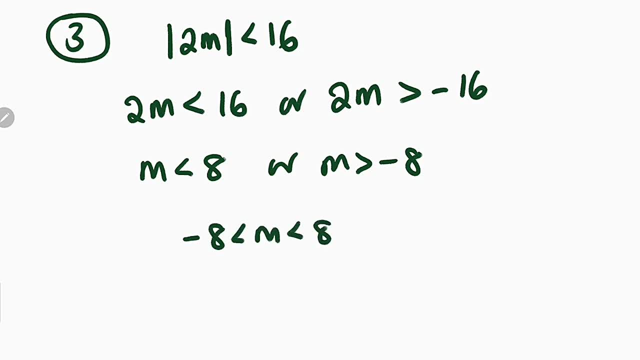 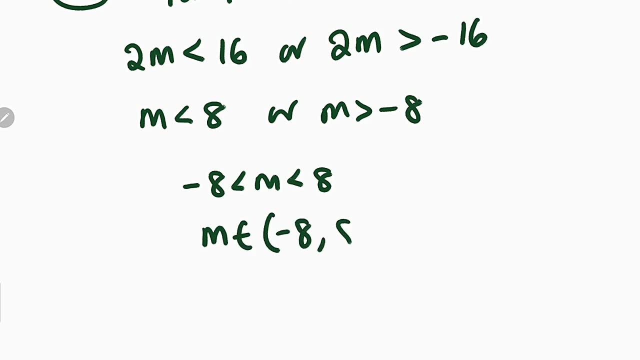 Negative 8, less than M, less than 8.. Or in an interval notation you say that M belongs to the set of values from negative 8 down to 8.. You You can also look at it on the number line, because you see we have 8 here. 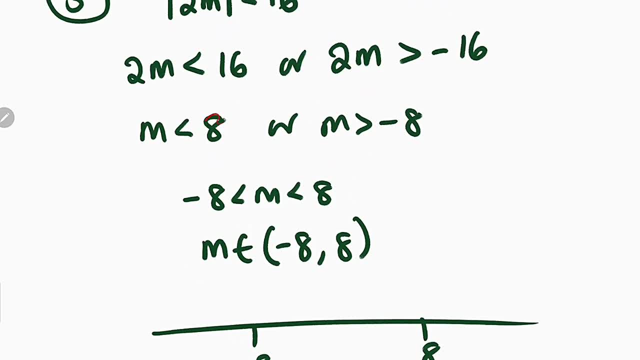 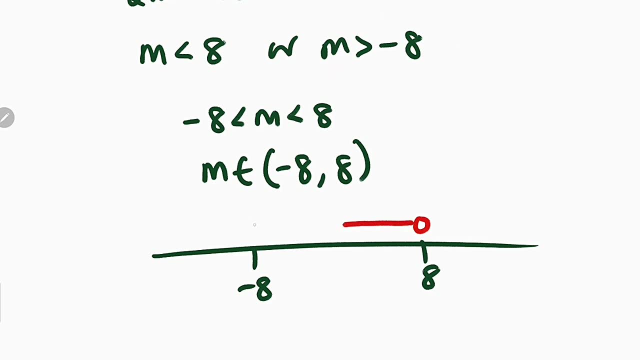 You have negative 8 here. So where M is less than 8, we are talking about these values. to the left, M greater than negative 8, we are talking about these values. So we have a solution: from negative 8 down to 8.. 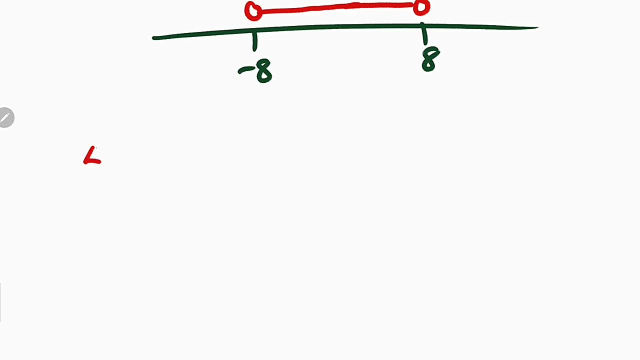 Let's take problem number four. So problem number four, we have the absolute value of S minus 1. Negative 15 is greater than negative 15.. There are some problems that you don't have to solve, Because any value in an absolute form will be positive. 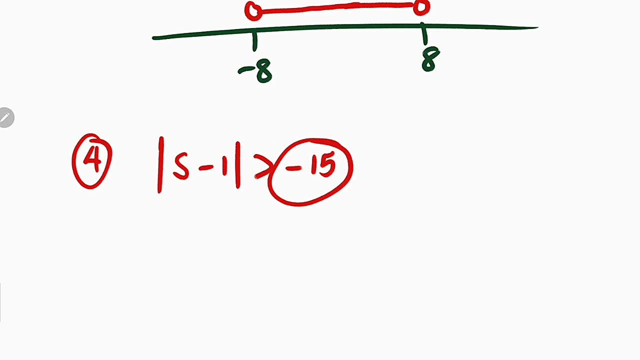 And all positive numbers are greater than a negative number, irrespective of whether it is negative 1 or negative. infinity Right. So this is always true, No matter what value plug in here. even if S is equal to 1, we have 1.. 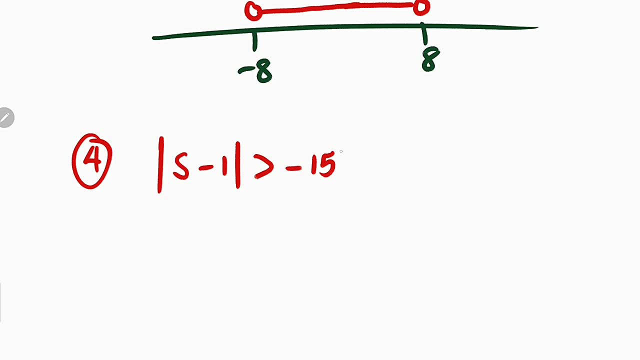 minus 1 is 0. absolute value of 0 is 0. 0 is always greater than negative 15. just look at it on the number line. we have a negative 15 right here. so any value you plug in here would be greater than negative 15, even if it is negative 16. if you plug in negative 16 here, it will be negative 16, negative. 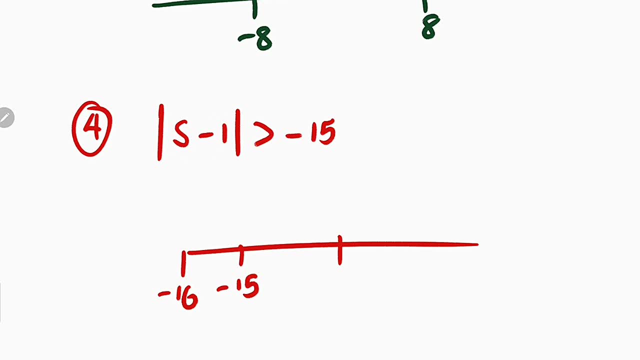 1, which is negative 17. an absolute value of negative 17 is positive 17, and positive 17 is greater than negative 15. so we conclude that s here belongs to the set of all real numbers. this is the solution to this problem. let us move on to question number five. 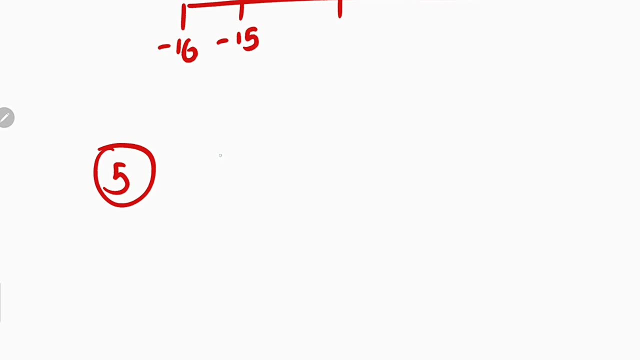 question number five: we have the absolute value of a divide by four, less than a or equal to 19.. first of all, we cross multiply. take four, multiply by 19, that will give us 76. so we have the absolute value of a less than or equal to 76. 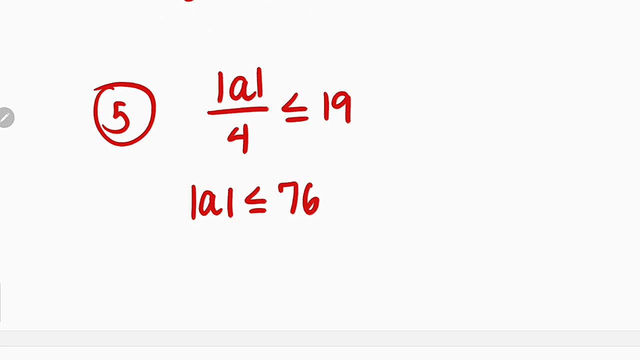 remember that this could be negative or positive, right? so, um, a could be less than or equal to 76, or you take a, you negate this one, you change the direction and negate this one to negative 76.. So this is the solution. So you can write it as negative 76. 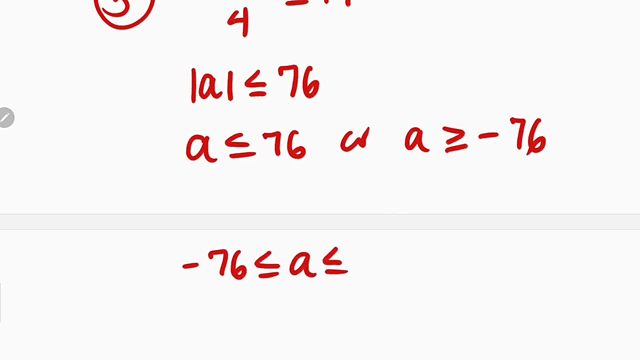 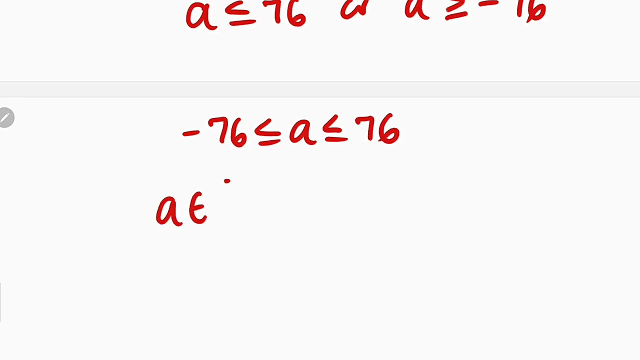 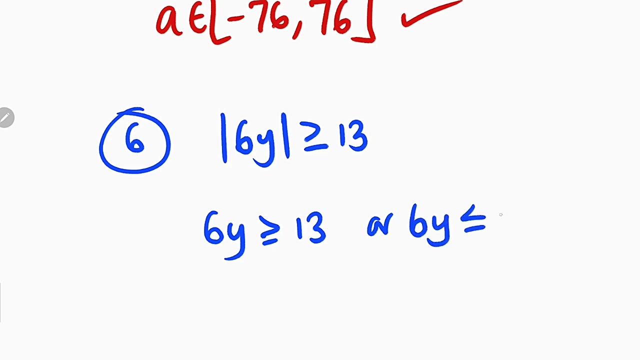 down to positive 76.. On an interval notation you see that a belongs to the set of values from negative 76 down to positive 76.. Let's move on to number 6.. Number 6, we have the absolute value of 6y greater or equal to 13.. So this 6y is either greater or equal to 13, or 6y is less than or. 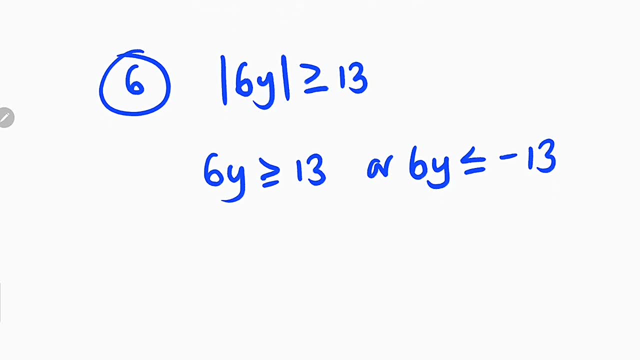 equal to negative 13.. So this 6y is either greater or equal to 13, or 6y is less than or equal to negative 13.. You divide both sides by 6.. y is greater or equal to 13 divided by 6,. 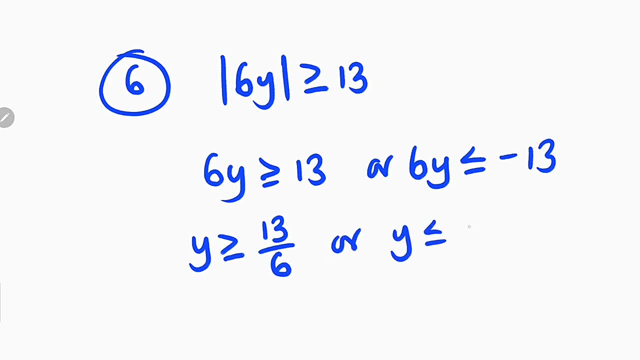 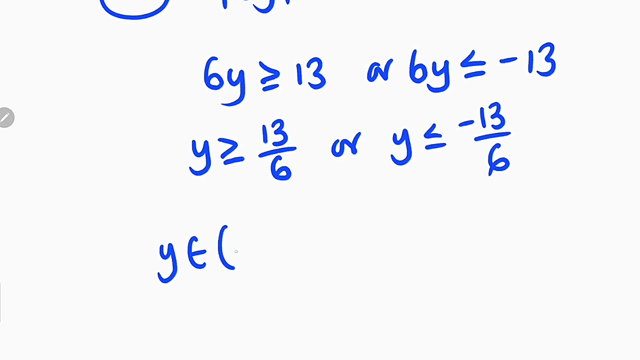 or y less than or equal to negative 13 divided by 6.. So you can write it in an interval notation, as y belongs to the set of values from negative infinity down to negative 13 divided by 6, inclusive. This magnification here is the total value of the absolute. 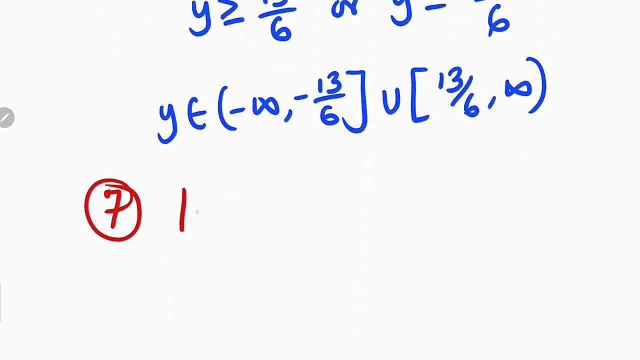 Moving to number 7. We have the absolute value of negative 7 plus r, and this is greater than 17.. So it is negative 7 plus r. Nos thi s reply: R greater than 17, or negative 7 plus R, less than negative 17.. You take negative 7 to the. 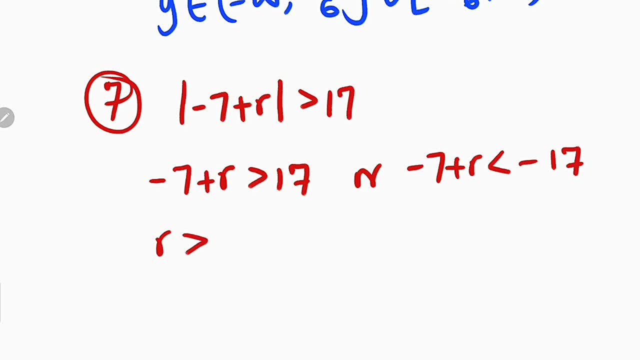 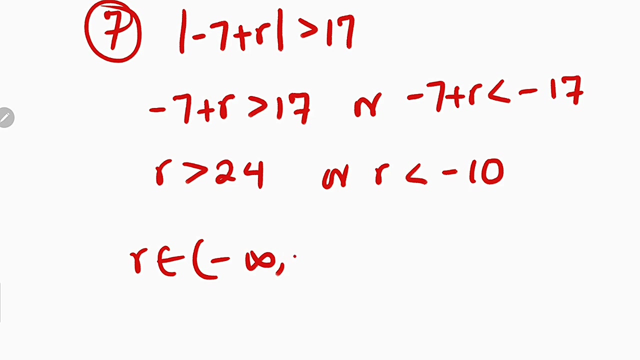 other side, it becomes positive. 17 plus 7 is 24.. Or you take negative 7 to the other side, it becomes positive. So R is what Less than negative 10.. So this is the solution to this problem. R belongs to the set of values from negative infinity down to negative 10. 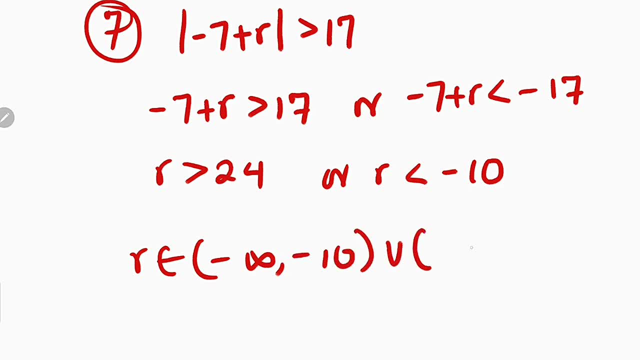 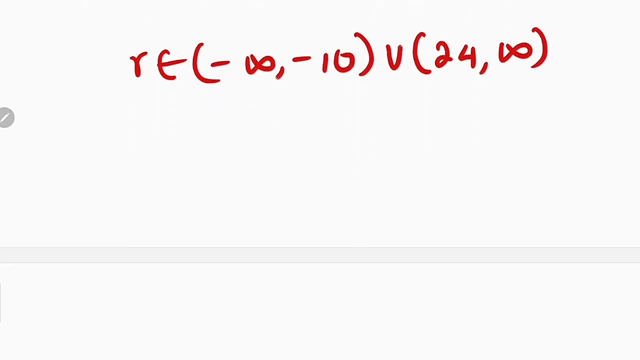 and union from 24 down to positive infinity. Let's move on to number 8.. We have the absolute value of U? U divided by 9, less than 20.. Multiply by size by 9, you have the absolute value of U less. 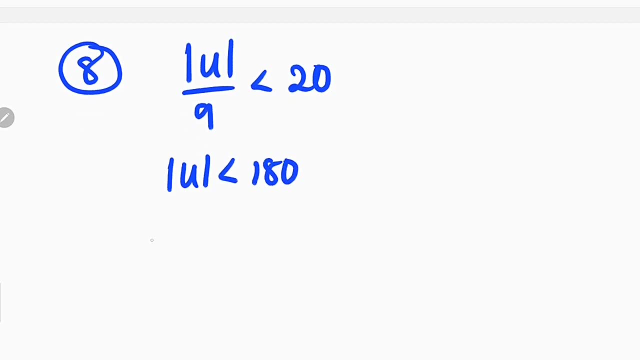 than 180.. You split it as U less than 180 or U greater than negative 180. So the solution would be from negative 180 down to 180.. Let's move on to number 9.. We have negative, the absolute value of 5Z greater or equal. 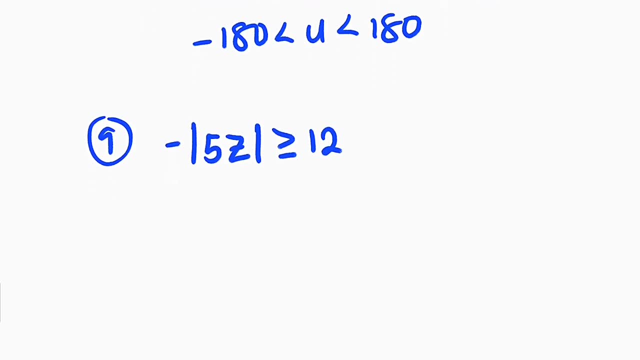 to 12.. So how do we go about this one? First of all, we have to get rid of this negative sign by dividing by size by negative 1.. So we have the absolute value of 5Z. If you multiply by negative, the direction of the inequality will change, So it becomes less than or equal. 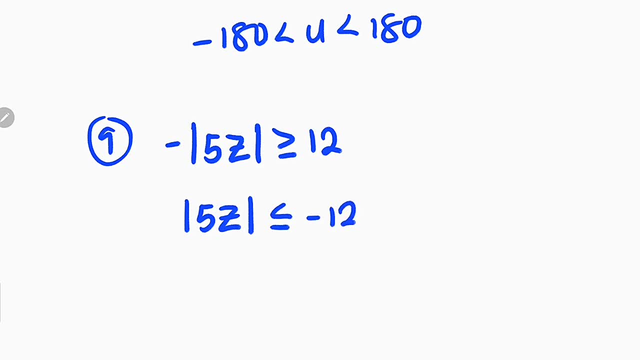 to negative 12. You don't have to solve this problem because you know that this is always positive And there's no way a positive number will be less than negative 12. So no value of Z will ever satisfy this problem. So we say that Z is what Empty. How do we write? 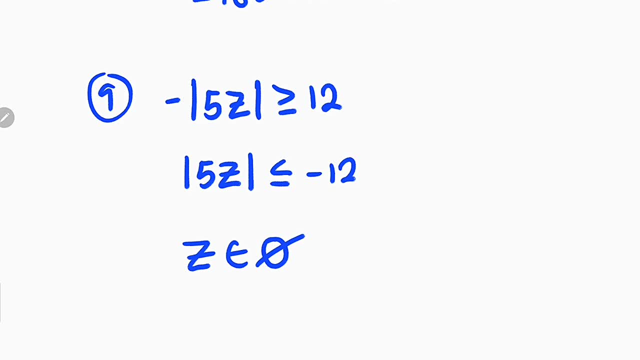 it like this: Z is empty Number 8.. For 10, we have the absolute value of negative 10n greater than 14.. So negative 10n is greater than 14, or negative 10n less than negative. 14 divide by size by negative 10, so n is less.